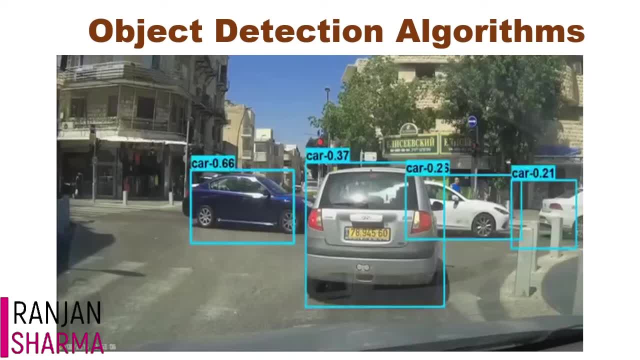 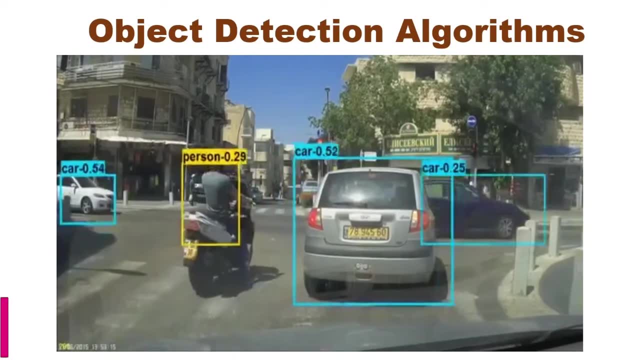 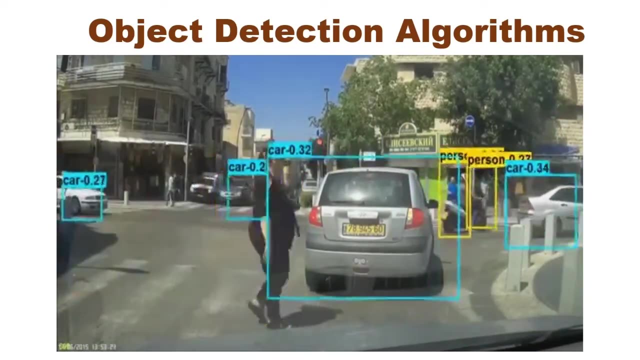 detect almost any object, or from the given image or video or real-time moments, and we can detect any type of the object to the very minute details, such as brand name of the car or a logo on the car, or we can detect anything. and the interesting thing is that there are many pre-trained models. 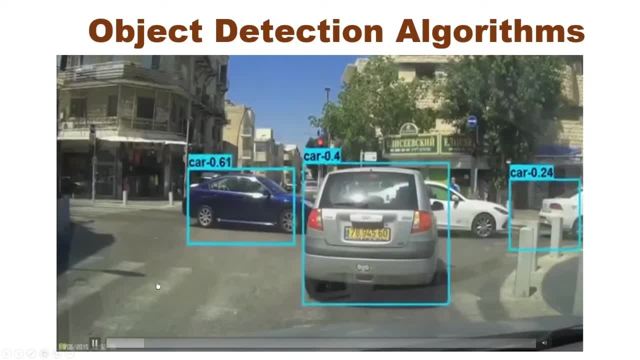 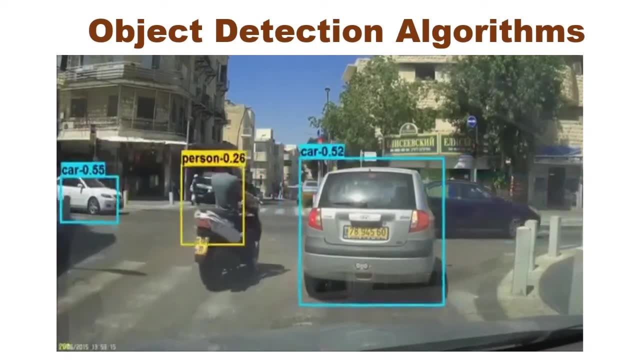 which are available in the internet, so we don't need to train each and every category of the object and that model we can use by some lines of code and i would be showing you each and everything in this playlist. and it's all possible due to the deep learning or the availability of the. 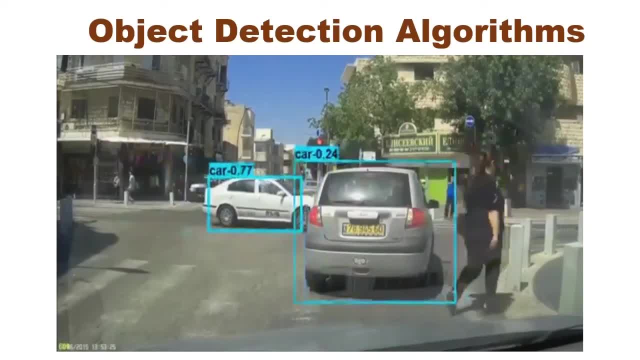 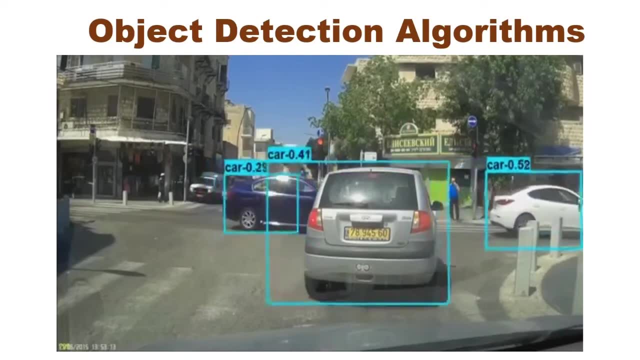 computation resources as of now, and i will be showing this implementation of such object detection in my third or fourth video. so in this video i will go through the foundation of the object detection, the basics of the object detection. i will be showing you what is the difference between. 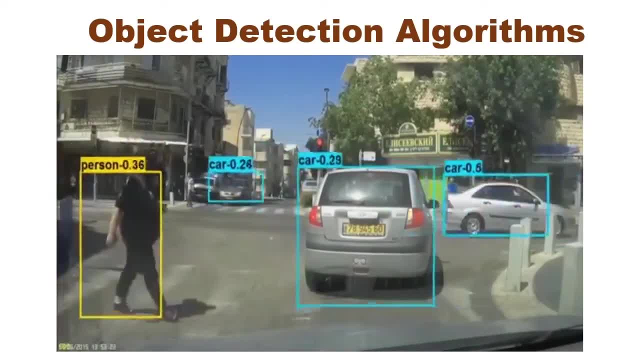 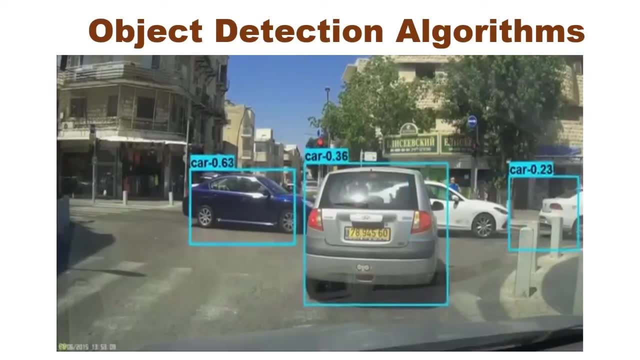 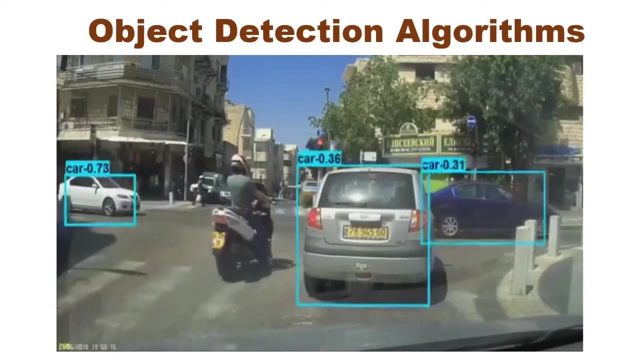 traditional object detection which we use earlier, like five or six years back, and now, what we are using now these days and what are the different stages in the object detection, how we trained and what are the some known state of the art models or trained model that we are using or we can say transfer learning. i will be show you some models. 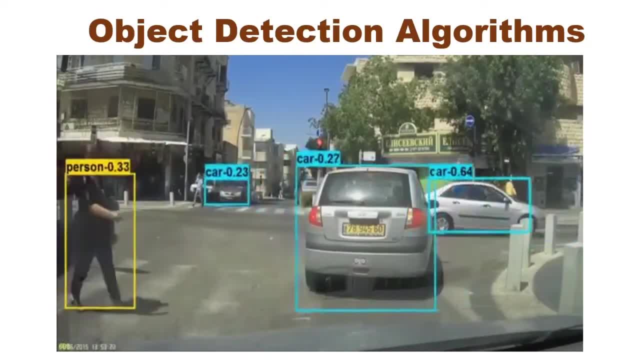 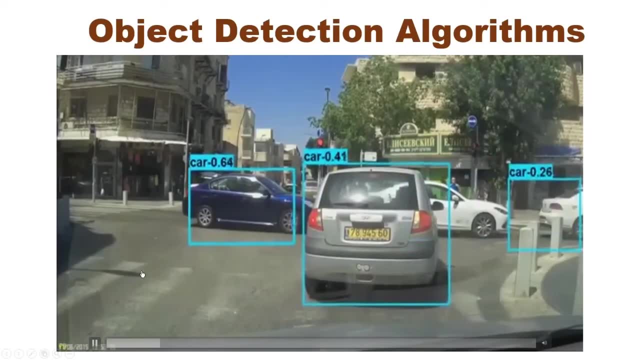 and what are the known data sets on which these pre-trained models are trained on and how we evaluate performance, whether our model is detecting fine or not, and if you already know about the bit and pieces and every basic of the object detection, you may skip this video. i will be uploading another. 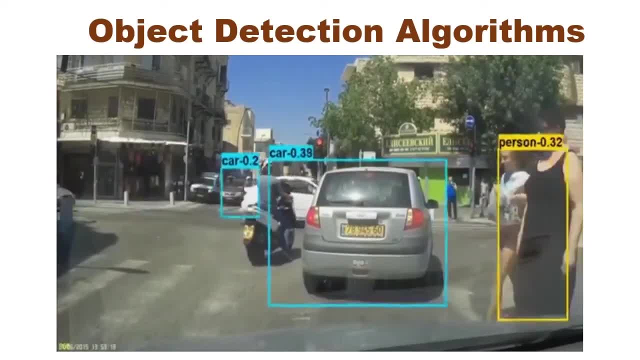 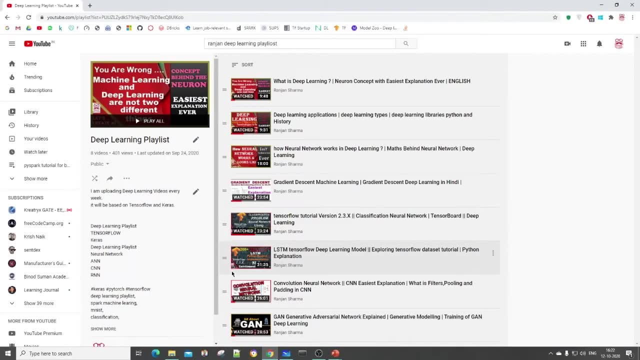 video for you guys. in two or three days you may refer that video for more advanced object detection. so let's start this video. and one more thing: if you don't know about the deep learning, if you don't know about the deep learning, just have a look on these videos that i have uploaded for deep learning. 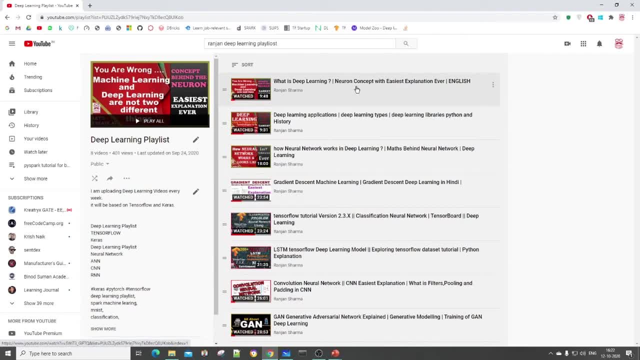 so in this playlist i have uploaded what is deep learning, how it works and what are the neural network, what are the types of the neural network and, second important thing, you should know about cnn, because object detection works on these two pillars, cnn and deep learning. so let's start this. 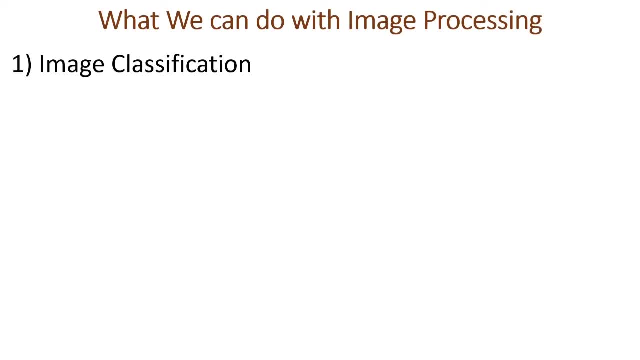 video without wasting any further time. so what is image processing? what we can do with the image processing? by processing image, first of all, we can classify the image, whether the given images of which type suppose we can classify. this image is cat, this is dog. so this is the first thing. 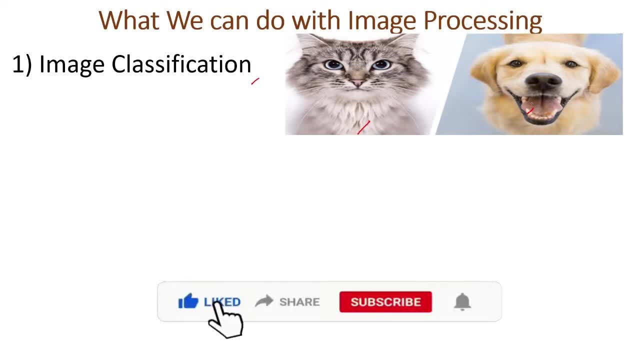 that we can do with image processing, so it's very easy in case of deep learning or machine learning. because it is just to classify. it's the case of only two images. it would be very quick to train on these two or three or four images, but it can detect. we will give some images of the cat and 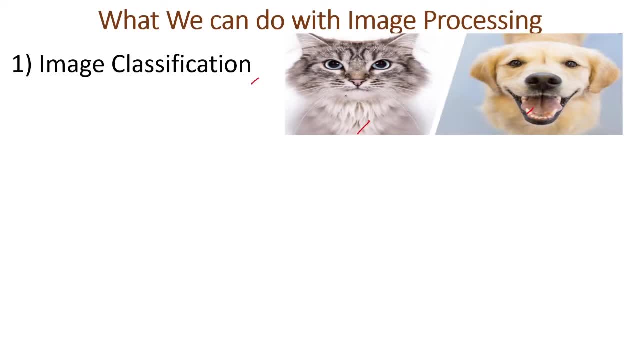 model with: yeah, this type of the image is similar to the cat, so this is cat. and second important thing is object classification and localization. so what is localization? if you will see in this image, it's there would be more background, but we have to detect in which part of the image our object is. 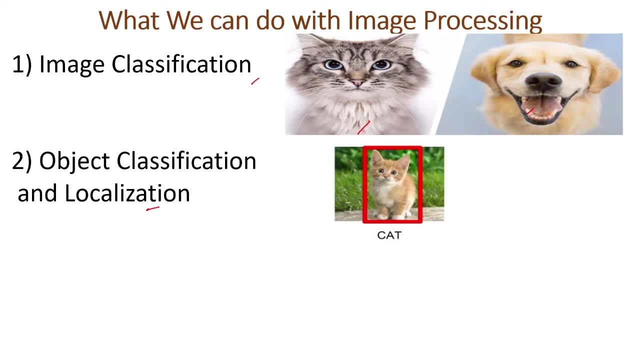 so this red line is localization, because if you will see, there is no cat, there is no cat, so this image is getting localized. so this is object classification and localization. so this is the type of object detection we can't say in this: this is a detecting a dog, it is classifying this. 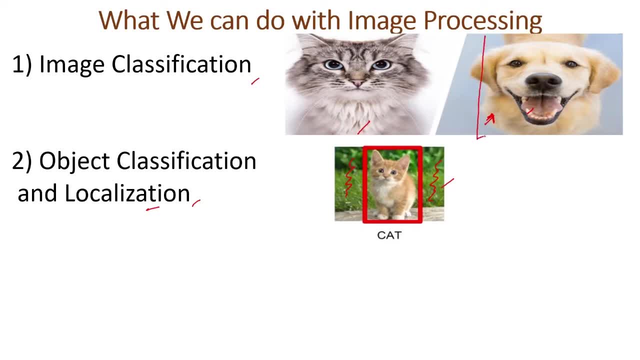 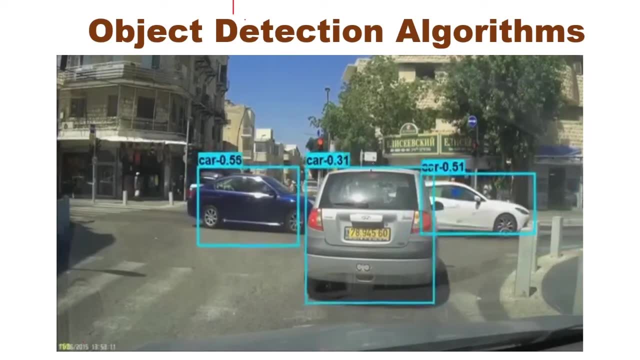 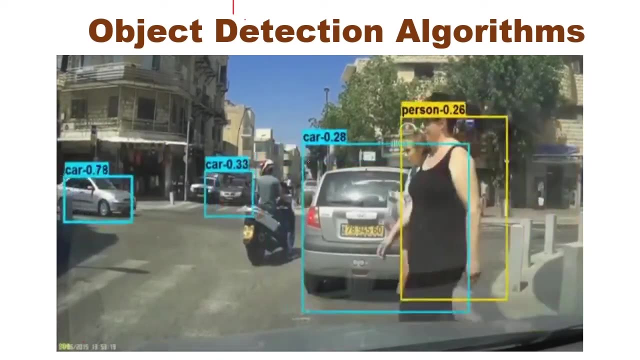 image into dog, but it is not detecting where the dog is, because dog is here. so this is bounding box. if you have seen in this image, you would be seeing a bounding box. so this is a bounding box. and here we have a percentage, this percentage confidence score. so this is object detection. 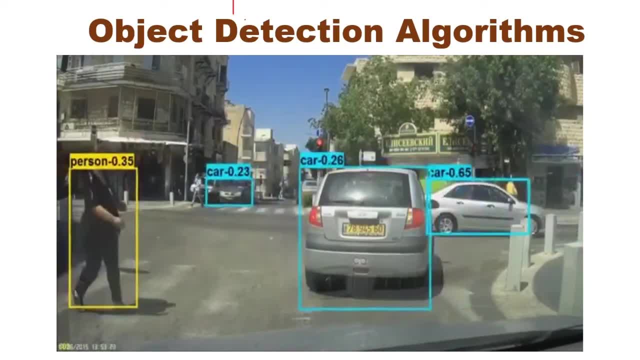 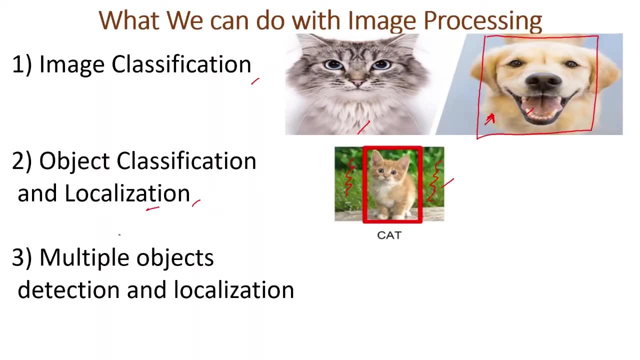 it is not classification, because it is detecting every object and it is localizing that object. so here you the same. so this is object classification and localization. and third thing is when we have a multiple objects in a single image, so we have to detect each and every object and we have to 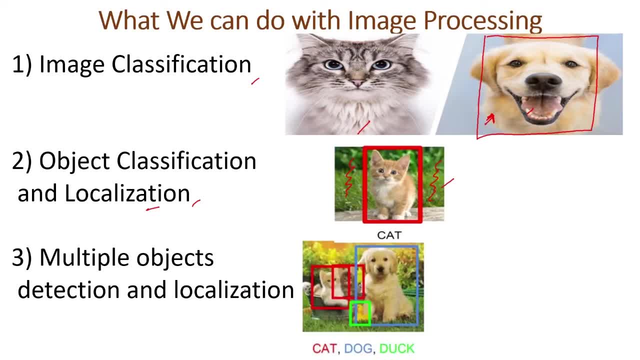 localize that object, in which part of the image we have an object. so if you will see, here we have dog, cat and duck. so it has localized that frame. so here we have dog, here we have cat, here we have another cat and here we have duck. so it has been classification and localization. so it has been. 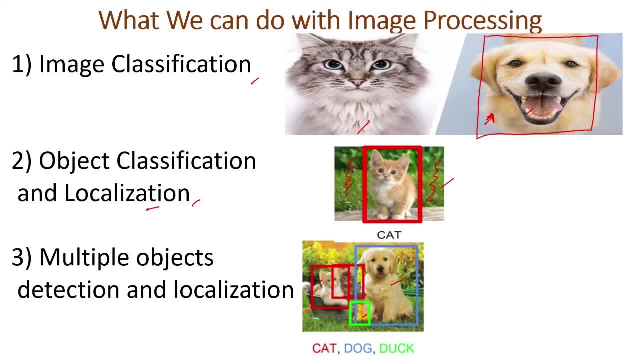 classified and localized and we have multiple objects. so these are the three important things that we can do with image processing, and it's not about only image processing. we can do with video processing in the real time video or a. we have a downloaded video. we can run the model on our video. 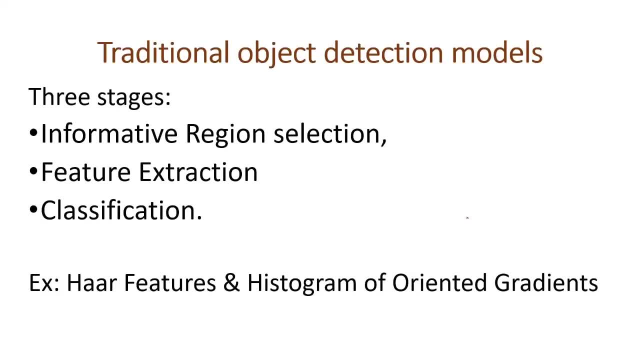 and it will detect which type of object it is. so earlier what object detection we are using, because earlier we don't had much GPU resources and computational resources, so we were not using deep learning, we was using machine learning at that time. so earlier the pipeline of the 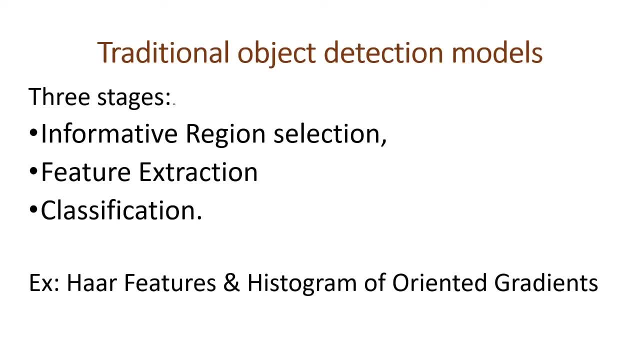 traditional object detection models has been divided into three stages. so first stage was information, region selection. informative region selection was that suppose we have a different objects in any position of the image. so we have image and we have different objects and in different region in the given image and it could be having different size. suppose here is a small. 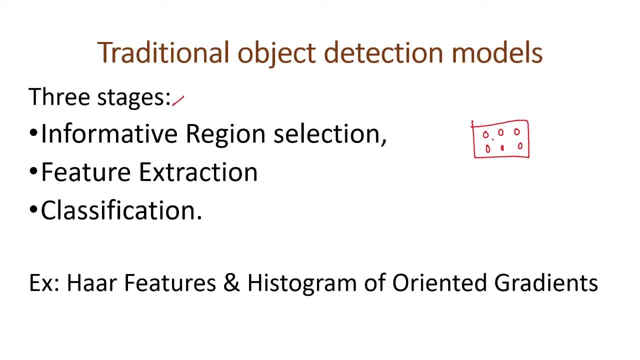 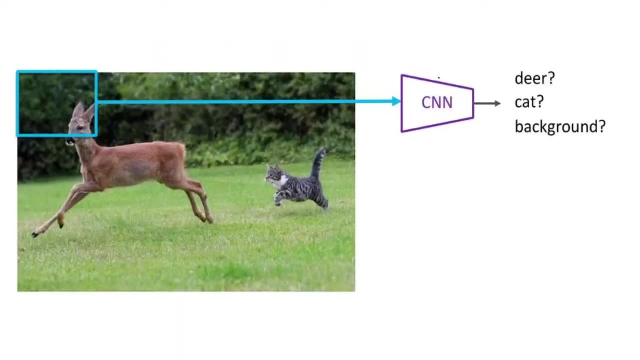 dog. here is a big dog and here a image of dog is there and it could be different aspect ratio or different size. so we have to scan the whole image with a multi-scale sliding window. so earlier we were using a sliding window. i will show you: in first stage we were using sliding window, so how? 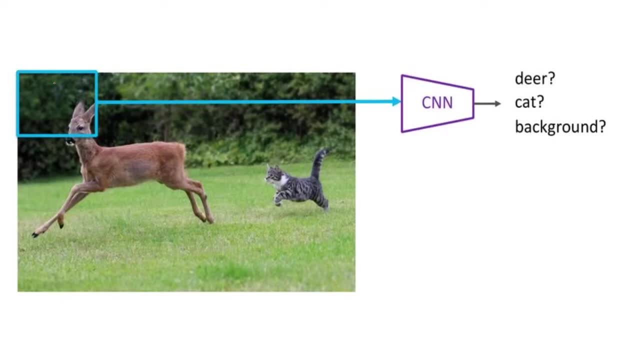 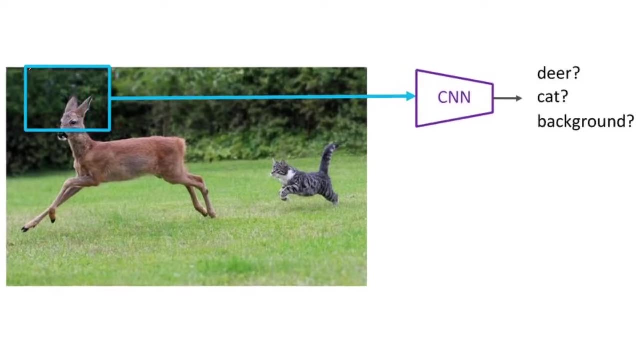 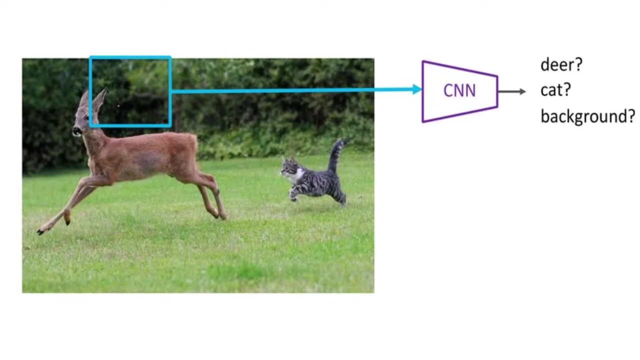 was that? so suppose this is a window and we have selected this side of the window. what we will do? we will slide this window to next level here, and it will be so here. my window has been slided to the right in the next level. it would be slided to this level, so we have to slide. 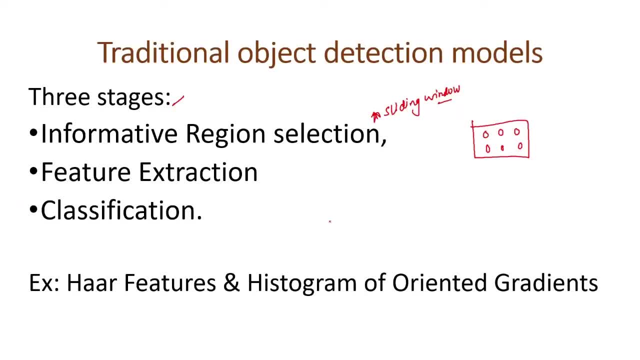 over windows to complete image. but this would be very exhaustive strategy to find out all the possible positions of the object, because what we are doing, we are capturing each and every part of the image by sliding, so obviously it will take computational resources. it would be very exhaustive. 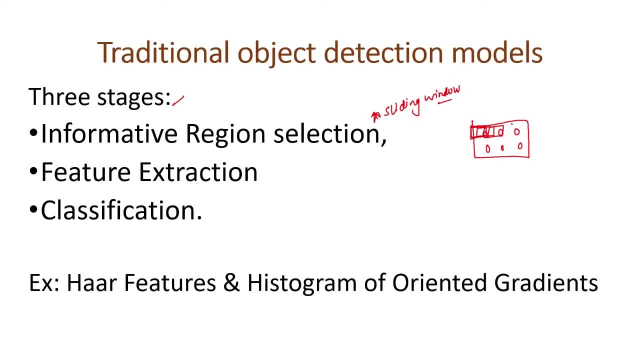 because it would be having a large number of windows. if we can do some customization, we can select fixed number of windows. but if we are selecting some fixed number of windows, suppose we have a image and we are selecting only six windows. so that would give us unsatisfactory regions because we may miss some more important regions. and once we have the 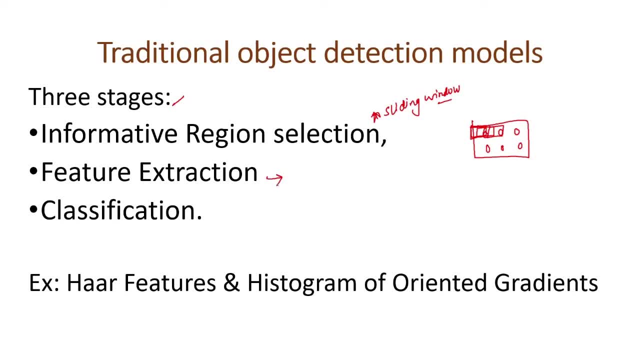 selected some regions here. then we apply feature extraction and as of now, these days, we are using cnn to do feature extraction, but at that time we were not using cnn. so what we are doing we were manually extracting features. so you could see that we were not using cnn, so we were not using cnn, so we 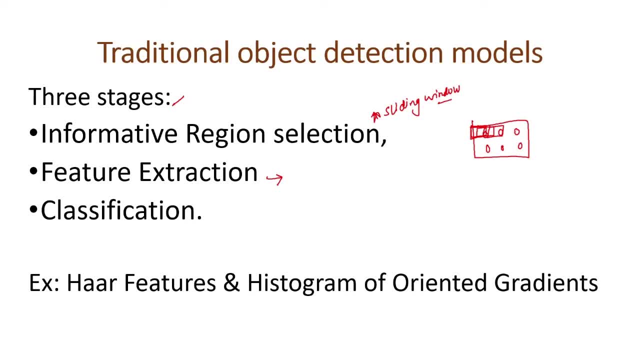 we have to recognize different objects that we have captured here. we need to extract visual features from the image which will provide a semantic and robust representation. that object is this, but due to the diversity- there are many appearance, illuminations, lighting conditions or background- it was very difficult to design a robust model. and once we have a feature- whether 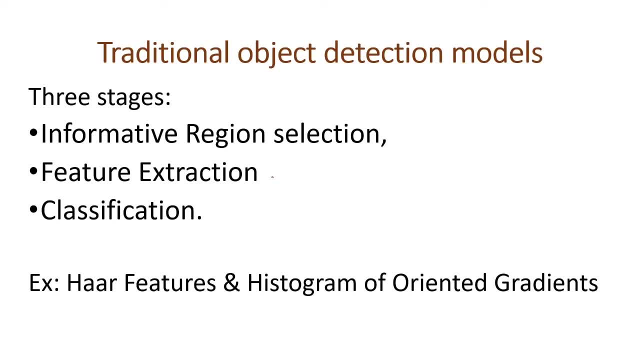 we were extracting manually or automatically by computer. then we were applying classification. so classification was that logistic regression or it could be support vector machine or would be add a boost, adaptive boosting. so this was complete machine learning. in this classification we were doing machine learning and example of the traditional object detection we we have already. 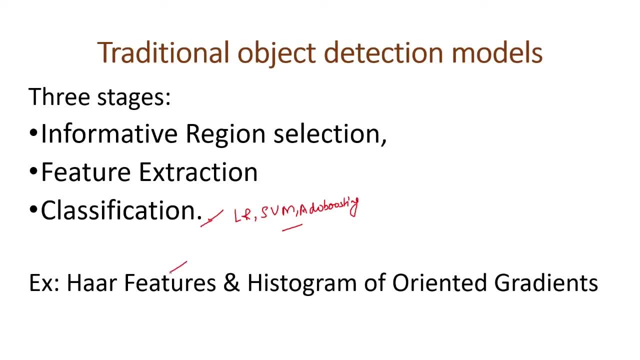 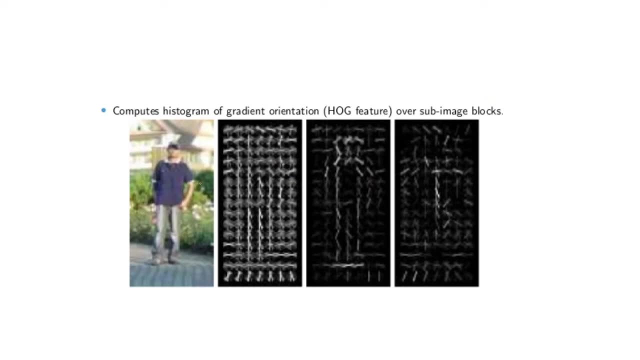 seen hard features. i have uploaded one video of computer vision using hard cascade features. in this video i have uploaded one video of computer vision using hard cascade features. if you have not watched this video, you can watch this video. here is a link and we have histogram of oriented gradients. i will show you. so this was a histogram of gradient orientation- what we are. 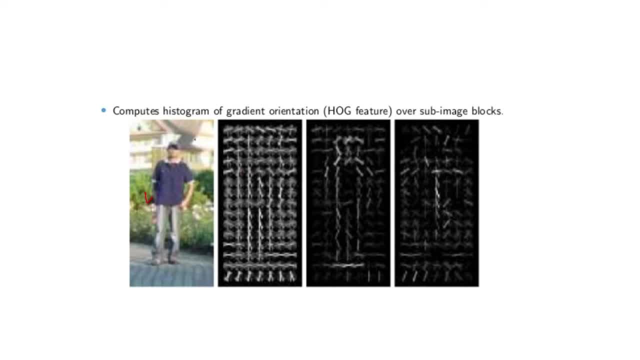 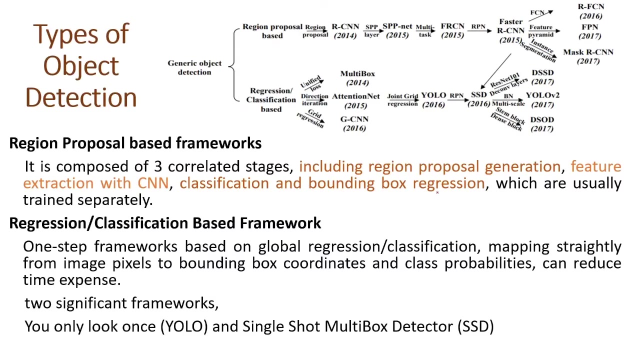 doing. suppose we have this image and we are applying histogram of gradient orientation and we are detecting some graphical representation. so in this graph you will see like this is representing a human-like structure. so it will detect this is a human. so now i will show you what object detection that we are using. 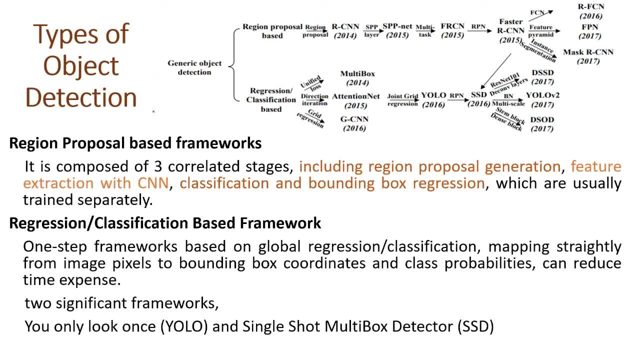 now. so basically, we have two types of object detection as of now these days. first is region proposal based. in this, if you will see, we have rcn and faster rcn, fast rcn and fcn, fpn or mask rcn. so these all type of region proposal based and this is regression classification based, multi-box. 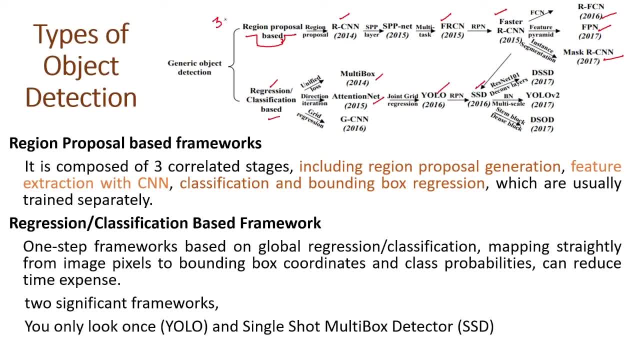 attention: net yolo ssd. this type has three stages and it would be of one stage. it would be a single step. it would be done in single step. it would be done in single step. it would be done in single step. so first we will talk about region proposal based framework. in this we have three things. first is 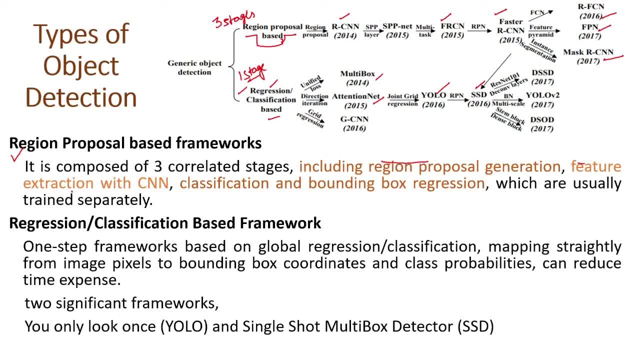 region proposal generation. second is feature extraction with cnn. and third thing, classification and bounding box regression. if you will see, it is pretty same as we do in traditional object detail, but in this we are using region proposal generation instead of information. region selection, in which we were using sliding window, but in this we are using region proposal generation. 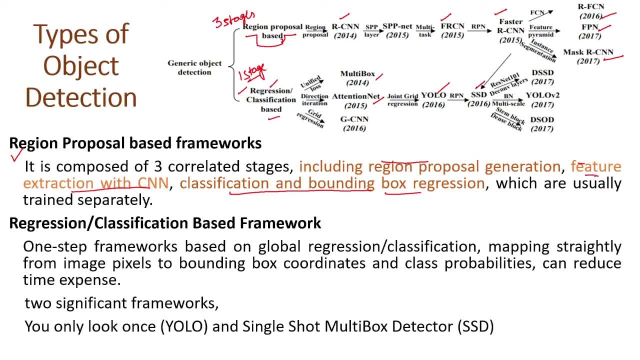 not using sliding window, and in second step, in that we were using feature extraction with machine learning, but in this we are using feature extraction with cnn. if you don't know about the cnn, you may watch this video. i have uploaded a video with a clearly explanation of cnn, so 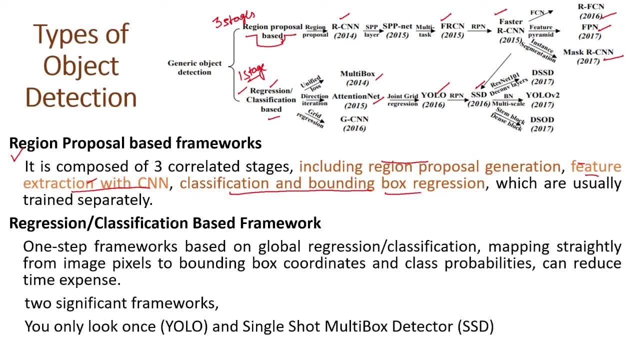 basically cnn is a convolution neural network and it's a neural network that has a special layer which is convolution layer or some pooling layers. and third is classification and bounding box regression. so bounding box regression is a classification and bounding box regression. so bounding box i have already shown you in the first video, a video with a object detection in which we have a. 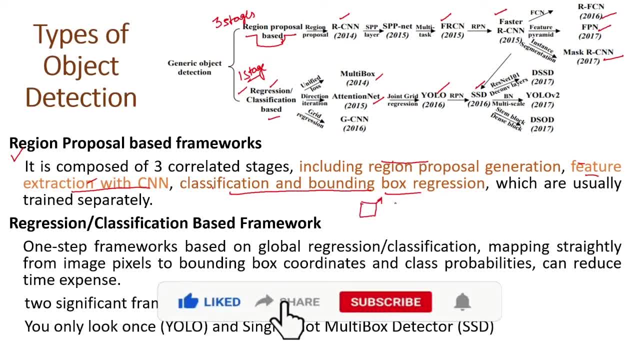 green color box. we say that as a bounding box. i will be showing you further videos. so regression, because it will calculate the exact plot of the bounding box. and classification, it will classify which type of category it is. so, and these three models usually train separately. we have to. 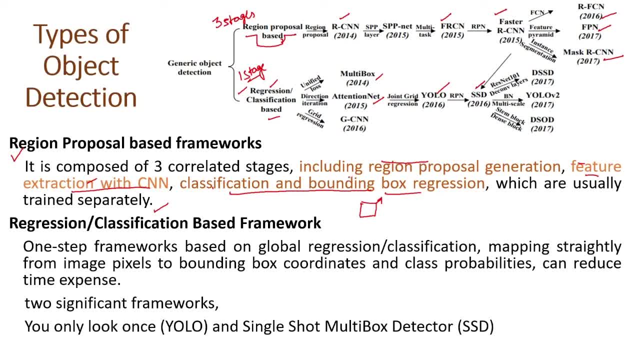 separately train these three models. so basically it has three models. so first i will tell you what is region proposal generation? these types of algorithm adopts selective search. selective search is a very important term because in selective search what it will do- suppose we have this type of image- it will divide this image into segment. now this image is having a number of 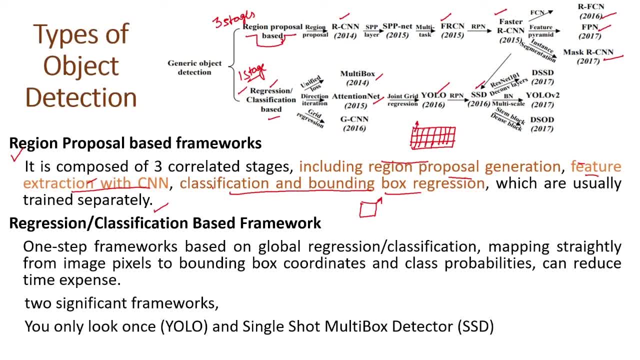 segments. every block is a separate region, so we are just generating a region here. so, basically, selective search method. it's algorithm that relies on simple selection. so that example is a segment that i will explain in a different video. but there are different ways of collecting different segments in a segment. so, for example, if i had a segment, 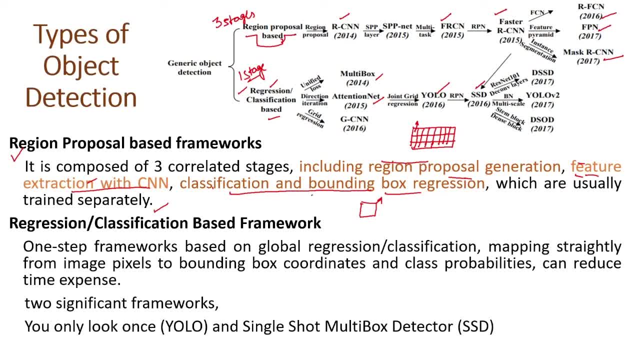 of the element which would be of the size of a reptile or a panther. so i can just click on segment there and it will allow me to select this segment. i will deploy one of my segments and i will apply some variety of segment. for example, i will show you panther or pattern. 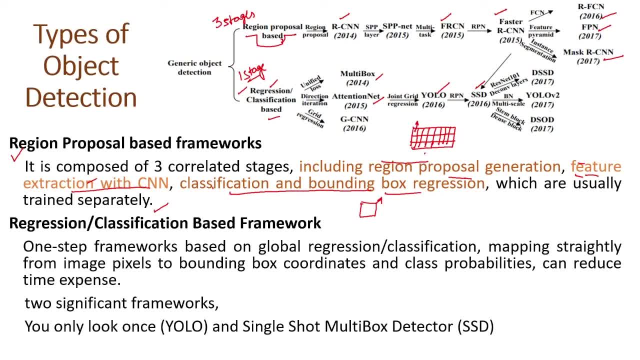 here we will apply different kind of types of segment, for example the panther, a pattern. here we are using non-pattern or pattern and i am creating a pattern in here. for example, i am using the pattern type in here, so i will apply some pattern. you will see that pattern. 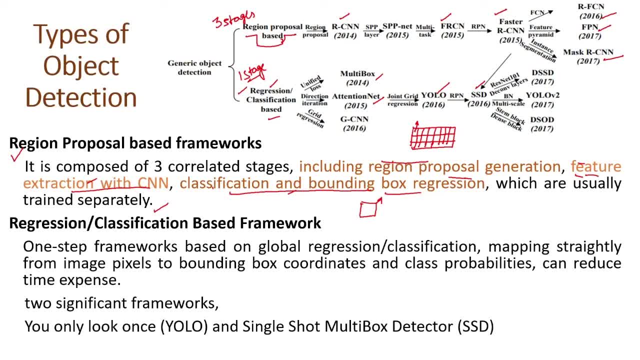 having some pre-trained category, so we would use linear support vector machine or we can use adaptive boosting for classification. so i will be showing you all these things in my next slides. so now we have regression classification based framework. if you will see, in this framework we were training three separate models. so basically it would be more time taking, so efforts would be. 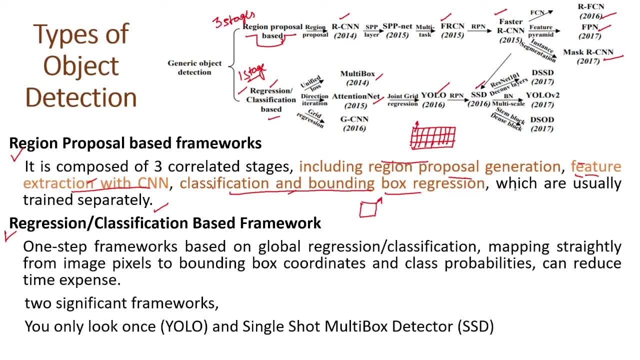 more and the time spent in the handling different, different components. it would be become the bottleneck in real-time application, because real-time application should be very quick. so that's why we have designed in a framework which would be completed in one step only and it would be based on global regression and classification. what it will do? it will just. 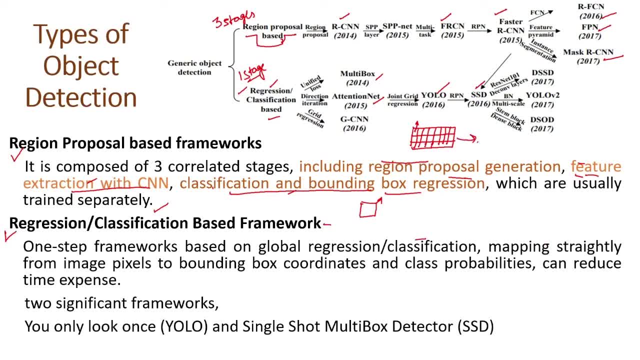 map straightly from the image pixels to bounding box coordinates and class probability. so it will reduce the time it is taking. so basically, it has combined all three things in one step only. so what it will do: it will just map straightly from the image pixel. these are the pixel and it will just convert to into. 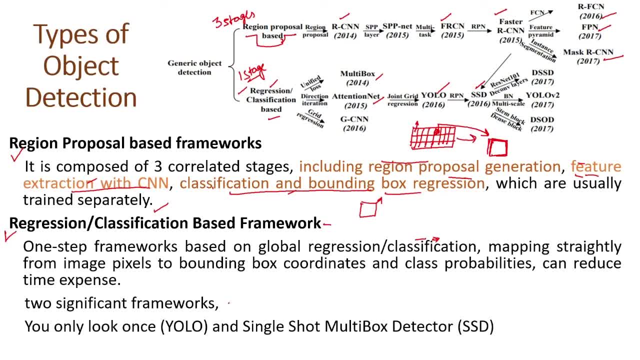 bounding box and we have two significant frameworks which we are using as of now. one is you look- you only look once, because it would be in one step- and second is single shot detector. so in this video, at this point, i have covered how was object detection earlier, when there was no deep learning. 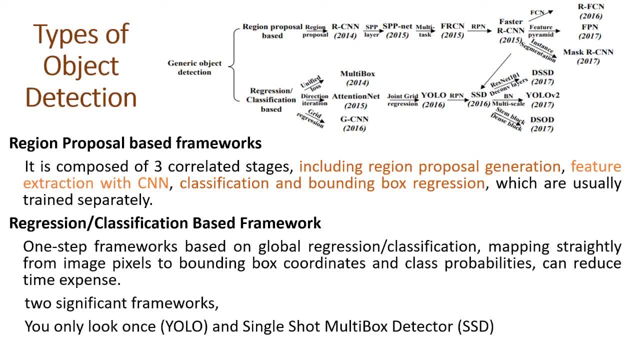 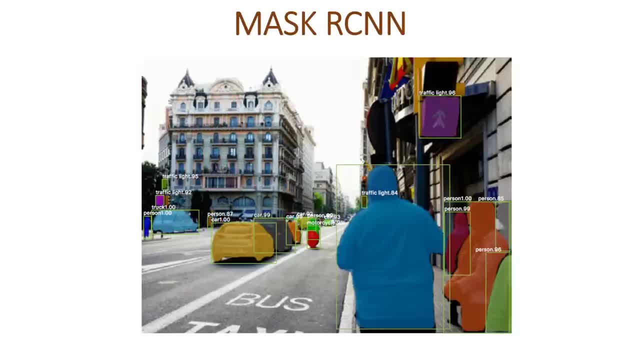 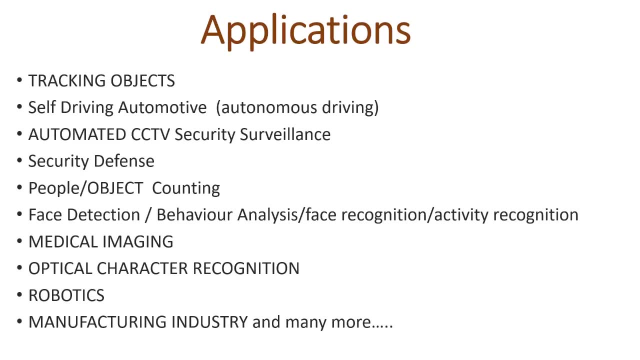 and how object detection is now and how it detects object. in the next video i will show you couple of pre-trained models, how they works, and then we will discuss some known data set on which pre-trained models are trained on. then we will see some annotations tool, then we will see application. so 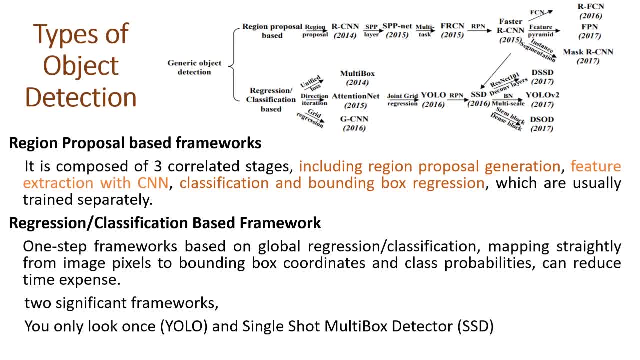 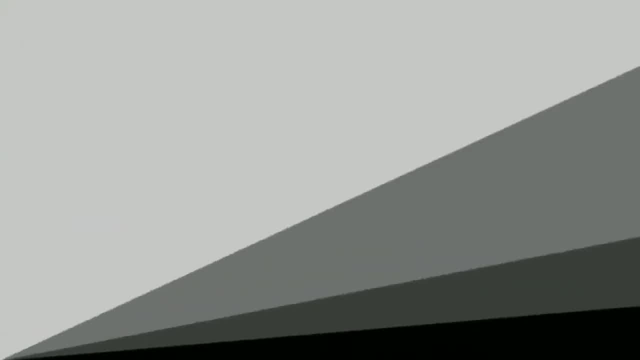 that's all in this video, so i believe you are interested to see more explanation about this topic. if yes, let me know. by posting the comment, i am giving my 100 to explain this topic. do let me know if i'm lacking somewhere or i'm missing something. to support my channel by subscribing.